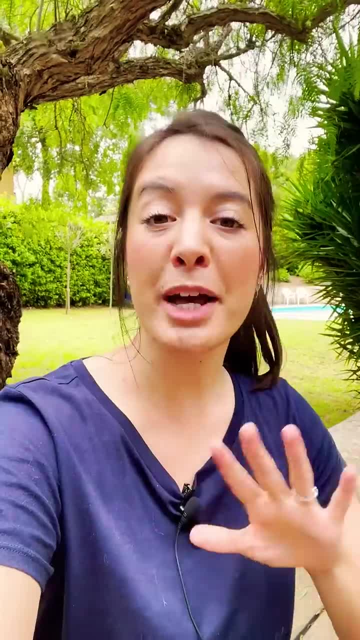 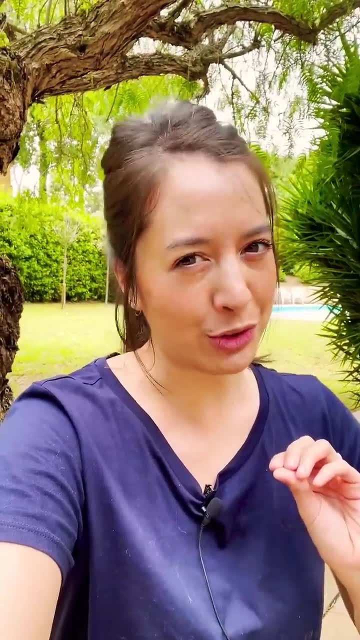 multidimensional sphere rather than deal with the equations, But by applying a branch of mathematics called complex analysis, Ahlisk managed to find the first exact solution, Although it's too complex for practical use. Problems like this remind us that complexity can be lurking in the most unexpected places. 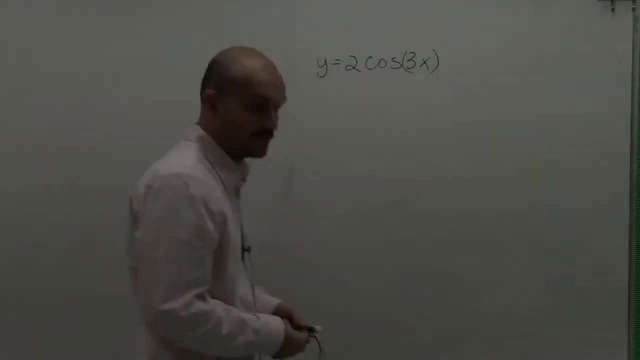 Welcome. So what I want to do is I want to show you how to find the period and the amplitude of a function, because that's going to be very important for us when we get into our graphing. So it's very important we get some practice on finding exactly what the amplitude and 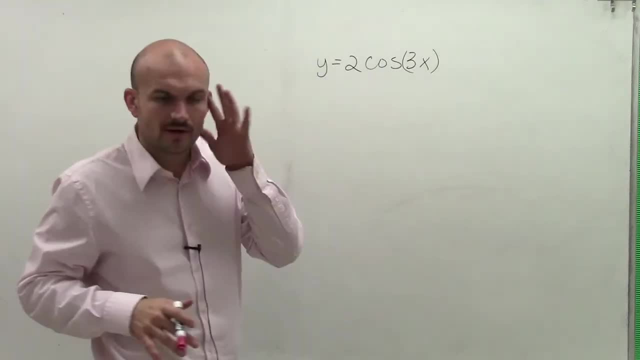 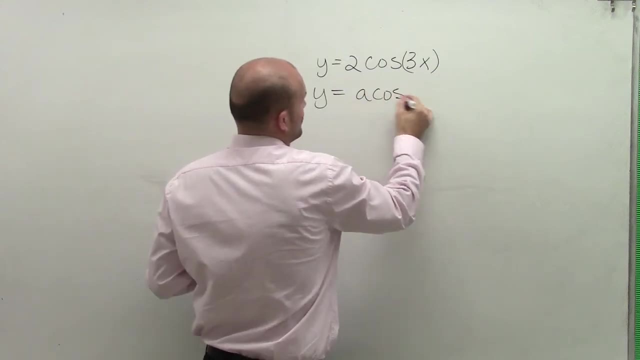 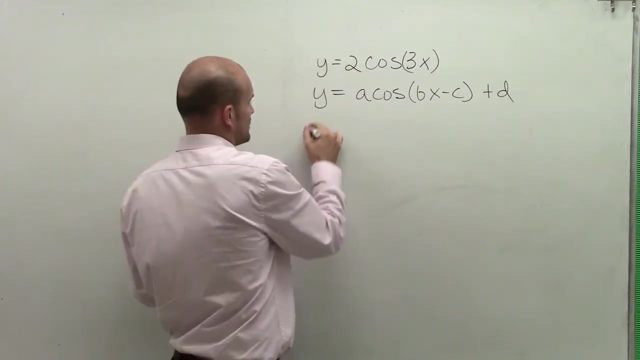 the period are. So first of all, when we have a function, we always want to remember what is kind of like our standard form of our function So we can write it in: y equals a times cosine of bx minus c plus b, And what we remember was the amplitude. Remember that was going. 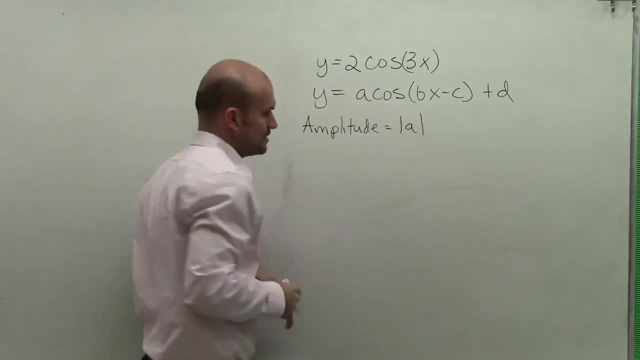 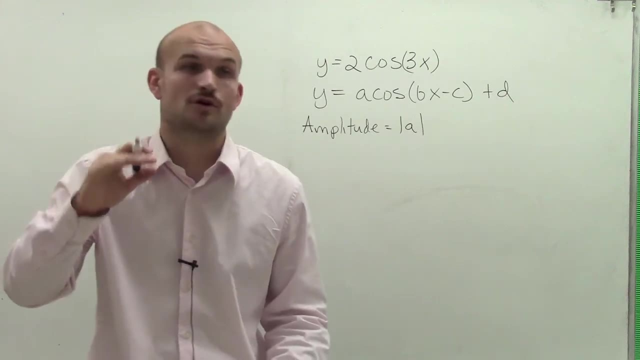 to deal with your absolute value of a. So remember, when dealing with the definition of amplitude, remember amplitude was the half distance between your maximum and your minimum of your graph. So to find the amplitude, we took the absolute value of our a And then 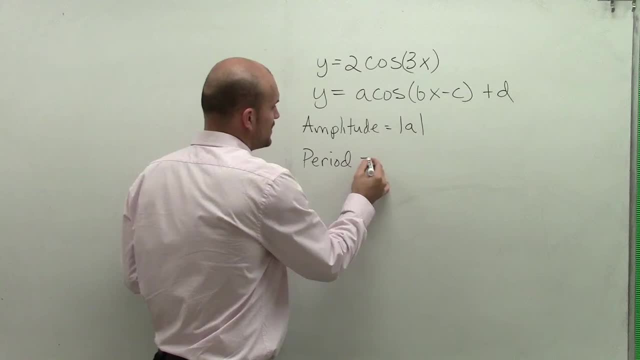 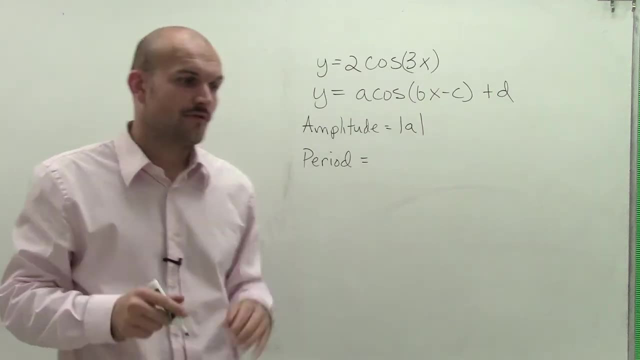 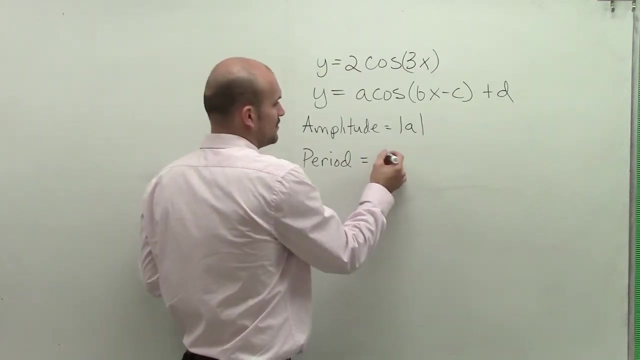 to find the period. Now, remember, the period of a function is the absolute value of a function. That was how far it took our graph to complete a cycle, for it to you know wherever it started, for it to go back to the exact same point where it started again. So we said our period. 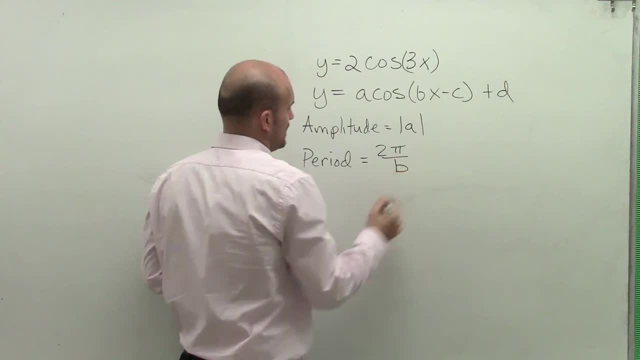 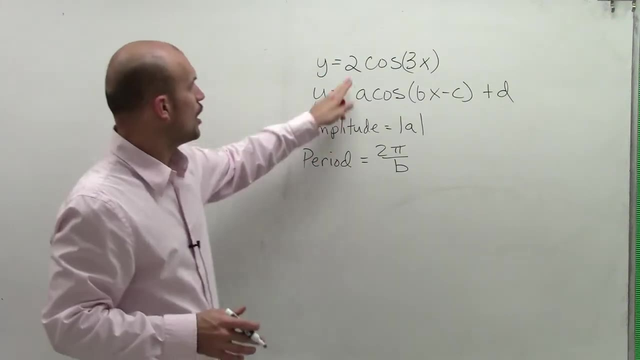 was always 2 pi divided by b. Now, when we look at these two definitions and we go back and we look at our function, we can easily see that our a, which is our number that's going to be multiplied by cosine, is going to be 2.. So the amplitude in this problem 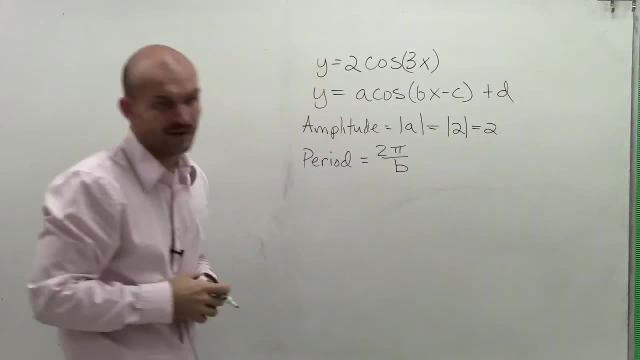 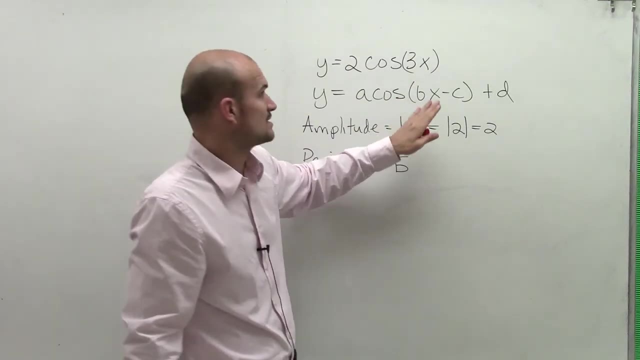 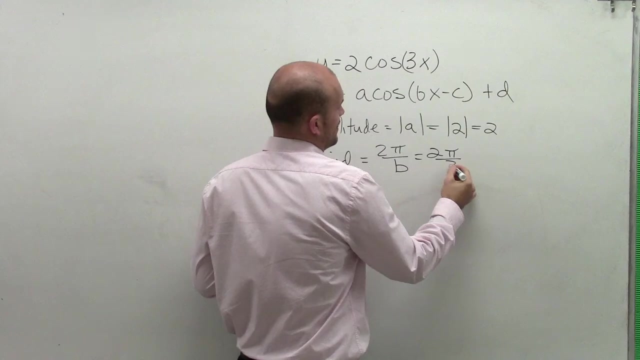 is the absolute value of 2.. Or we could just say it's 2.. Then the period we look at, the period, remember, is going to be your b, b is going to be your coefficient of x. So when we look at this, we say we have a, 3x. So therefore we could say: 2 pi divided by 3.. Well, we're. 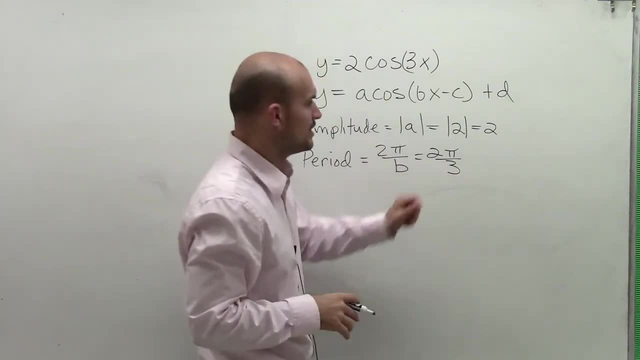 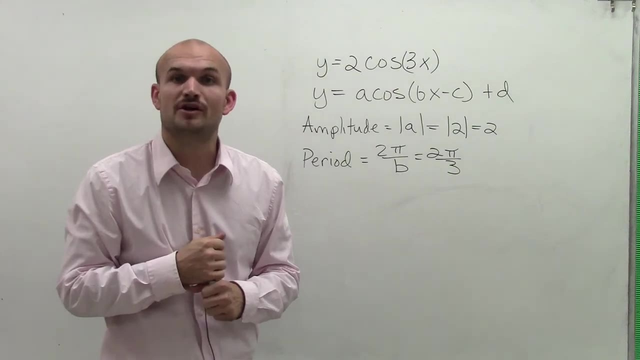 just going to leave that in that form. So, therefore, our period is just going to be related to 2 pi over 3.. So there you go, ladies and gentlemen. That's how you find the amplitude and period of a trigonometric function.